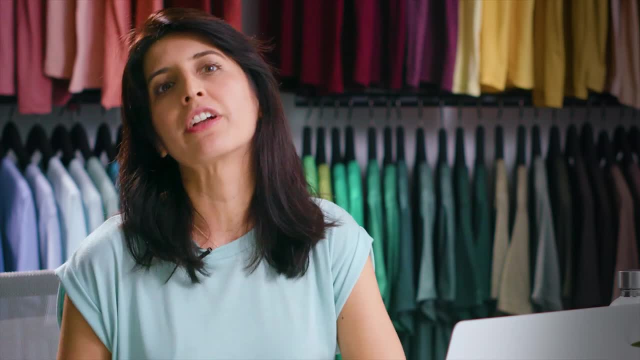 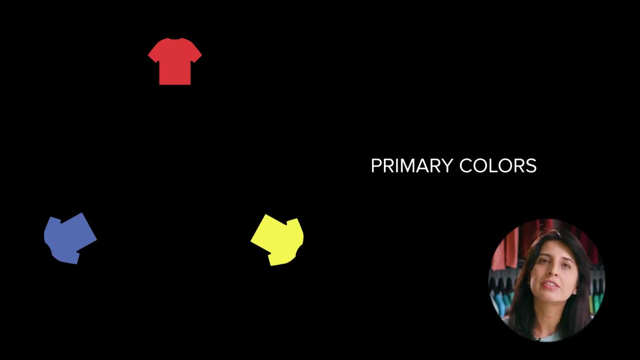 with the basics of color. There are two main categories for how colors can work together. These are primary and secondary colors. Primary colors are red, blue and yellow. Secondary colors are the colors in between the primary colors: orange, green and purple. If we mix primary colors, 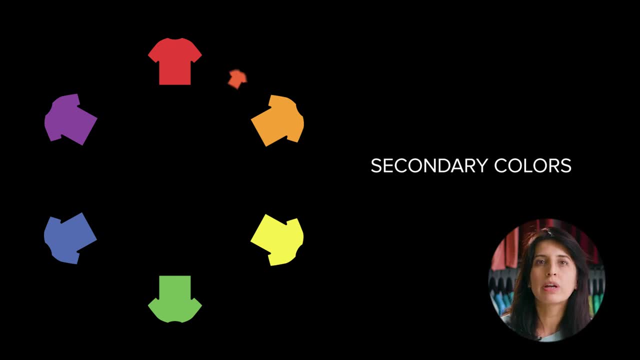 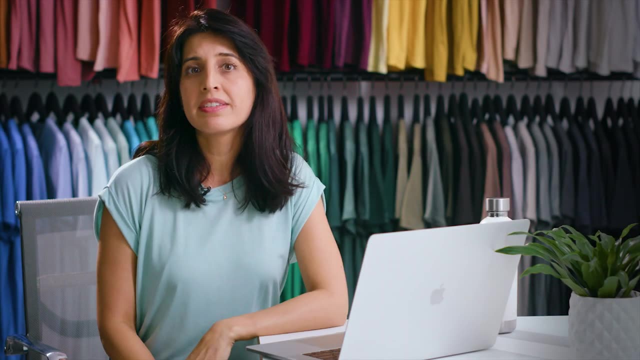 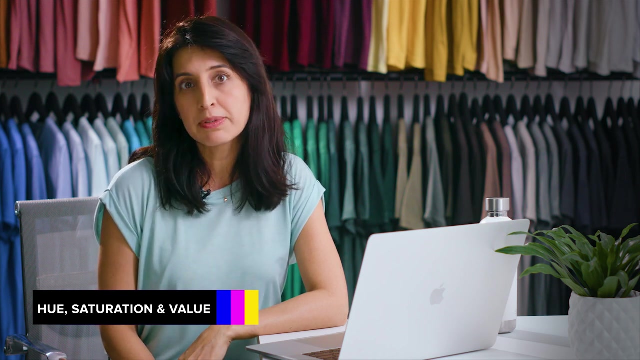 with secondary colors we get more in between shades like red, orange, yellow, green and so forth. Altogether they form what is called a color wheel. If we go one step further, we start to look at hue, saturation and value. These terms will help you understand more nuanced colors, like the little paint chips you'll find at. 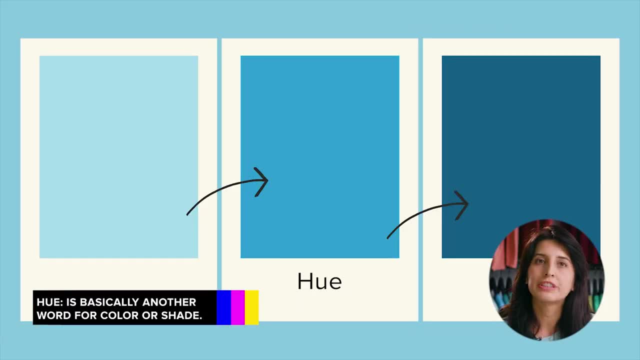 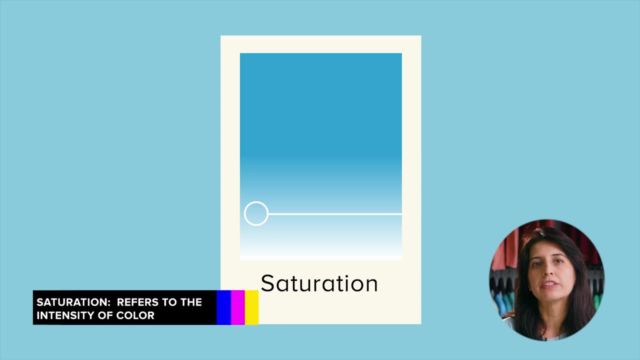 a home improvement store. Hue is basically another word for color or shade. Here are different hues of the color blue. Saturation refers to the intensity, in other words, whether the color appears more subtle or more vibrant. Highly saturated colors are brighter or richer, while desaturated colors 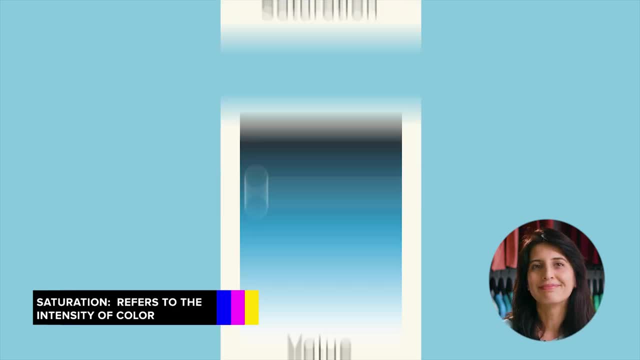 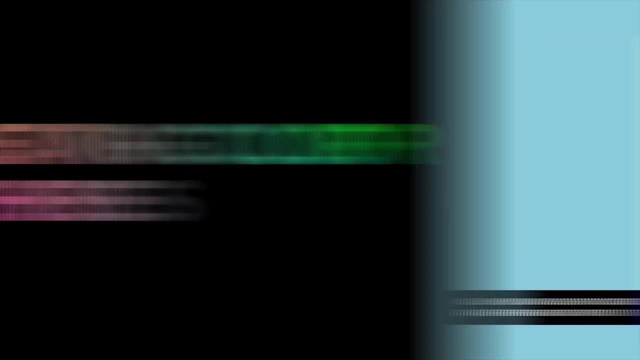 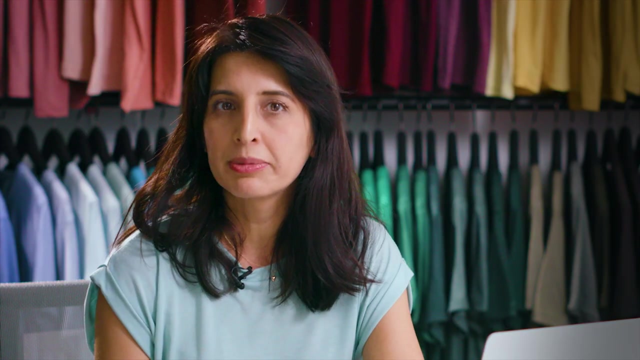 have less pigment. Here are different saturations of the color. blue Value has to do with how dark or light the color is, ranging from black to white. This gives us many different shades in between. So how do we put this all together to create professional looking schemes? There are formulas. 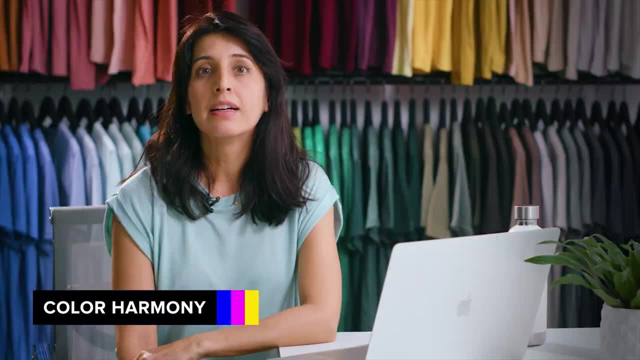 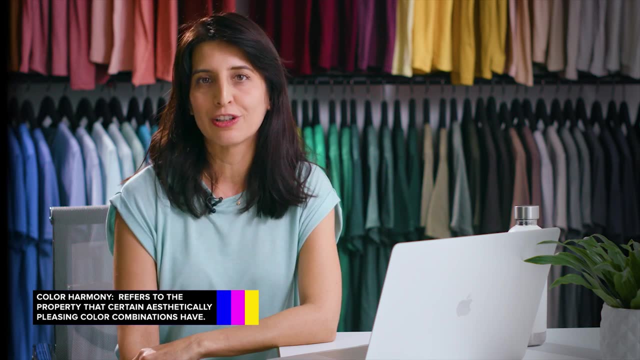 already created, based on something called color harmony that can help. Color harmony uses the color wheel to illustrate different color combinations. Some of the most common types of color combos are as follows: Monochromatic design is an easy way to form harmony, especially with your apparel. 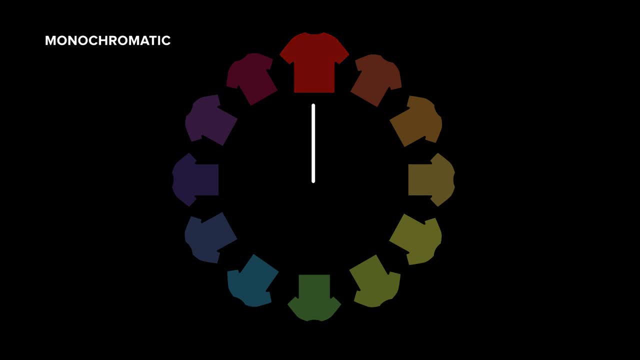 collection. Pick one spot color and adjust the saturation and values. You can also use making it lighter or darker to make different variations. When choosing this color scheme, you are guaranteed to match because the colors are all from the same family. You'll see this use of color on apparel from your favorite brands in retail stores today. Analogous color. 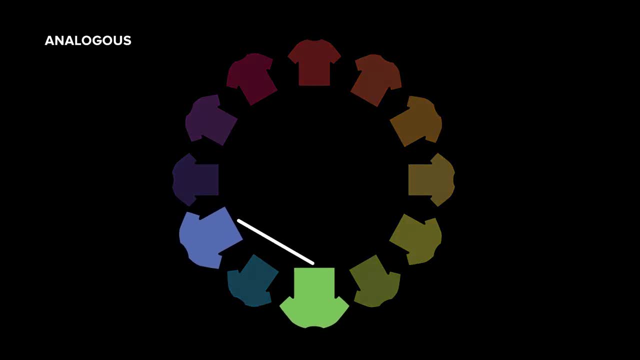 schemes use colors that are next to each other on the wheel, like blue and greens. Complementary colors are colors that are opposite each other on the color wheel, For instance red and green. You can add variety to these color selections by including lighter, darker or desaturated tones. 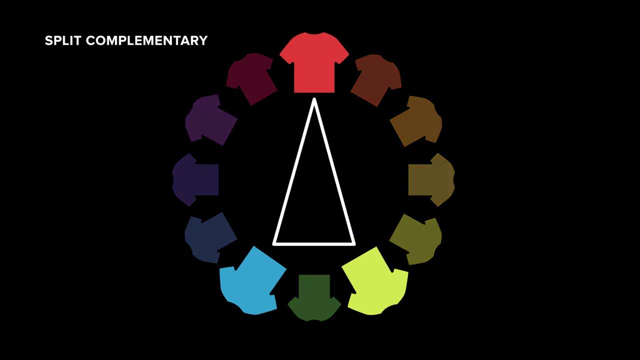 A split complementary color scheme uses the colors on either side of the complement. When using three colors that are evenly spaced on the color wheel, this is a triadic color scheme and it forms a perfect triangle. And finally, tetradic color schemes form rectangles on the wheel using two.